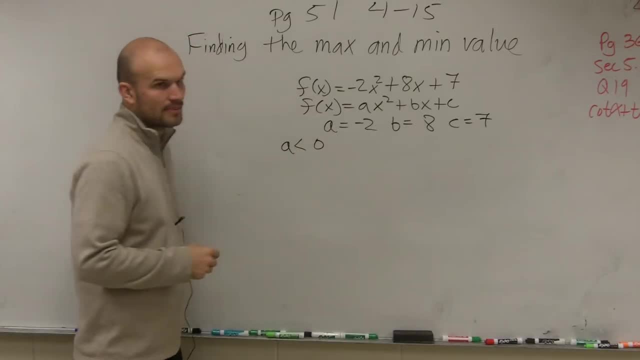 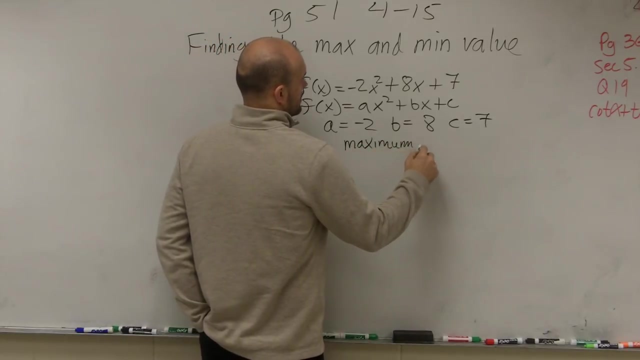 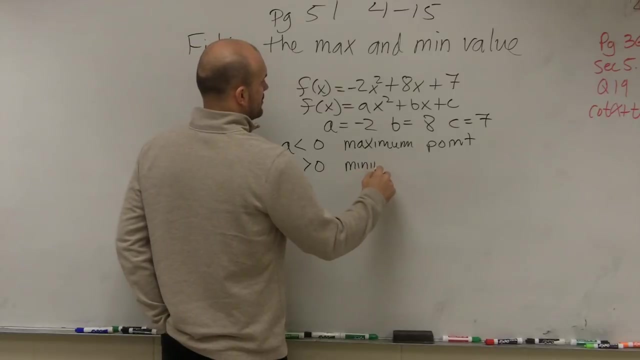 if a is less than 0, so if your a value is less than 0,, then you're going to have a maximum point, And I'll show you how to do that in a second. If a is greater than 0, that means you're. 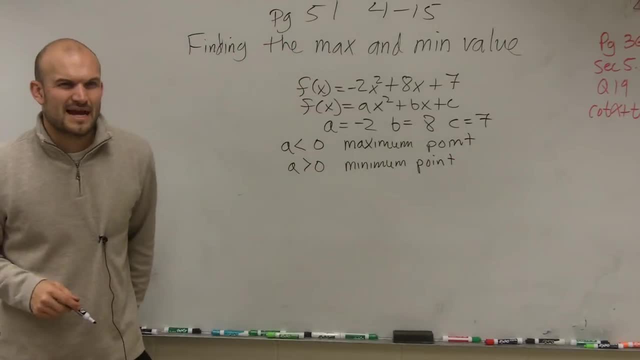 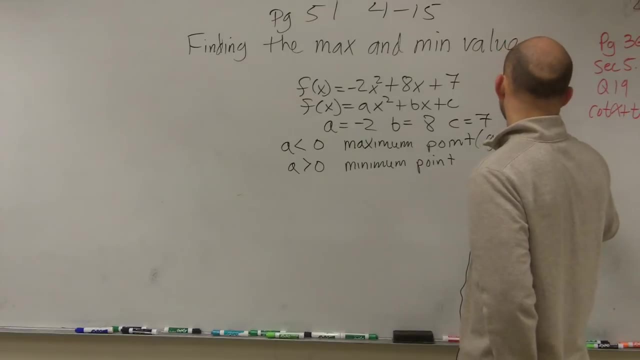 going to have a minimum point. And what does that really mean? a maximum or a minimum point? If you have a maximum point, that means your graph opens down, And if you have a maximum point, that means your graph opens up, alright. So what exactly does it mean? Well, ladies, 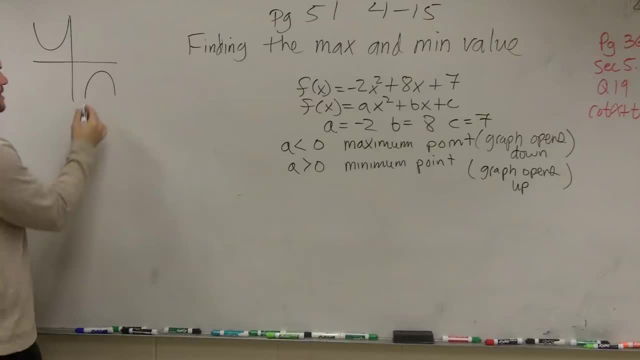 and gentlemen, the difference is this: Alright, we're talking about maximum and minimum points, So you guys can see if I have a point that's the minimum point, that's the lowest, my graph goes right. So that means my graph is going to open up If my graph has a maximum point. 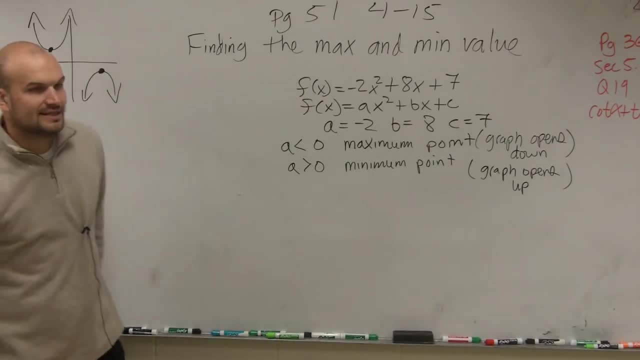 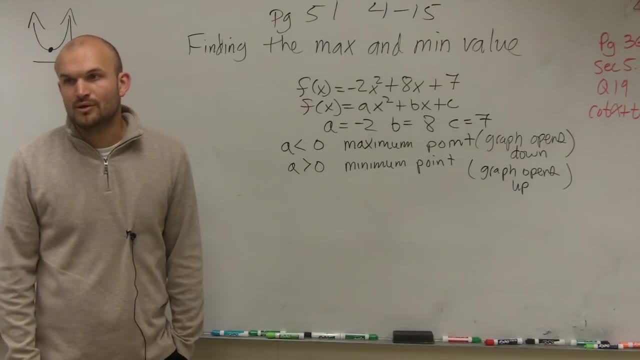 that means the graph opens down. So in looking at this equation…. So is my graph going to open up or open, or is it going to have a maximum or a minimum point? Maximum, Maximum point right A is less than zero because it's negative. two: 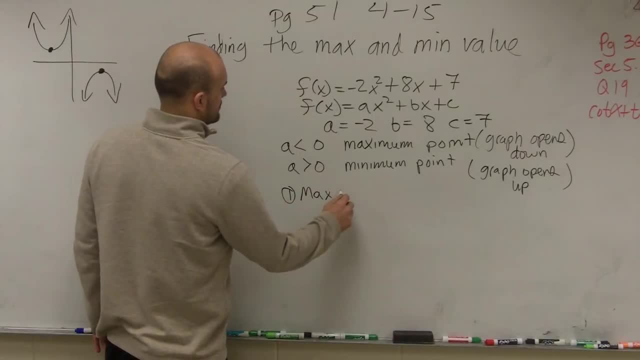 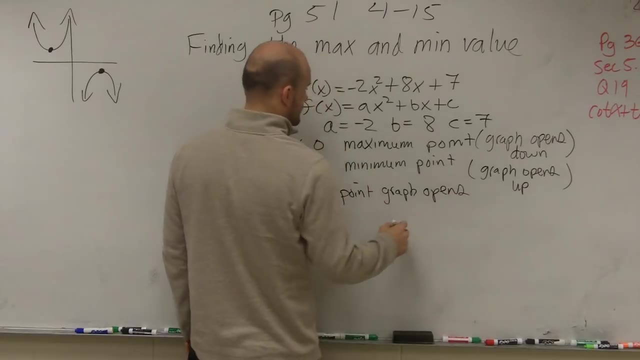 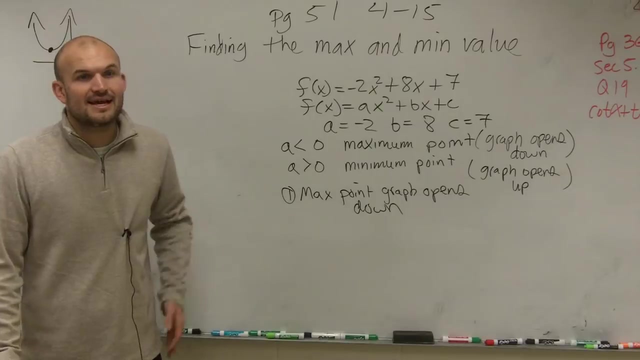 So, for our example, we have a max point. That means the graph opens down. okay, Now the next thing is it does say to find that point. So do you guys remember what is this point? do you guys remember what this point we call? 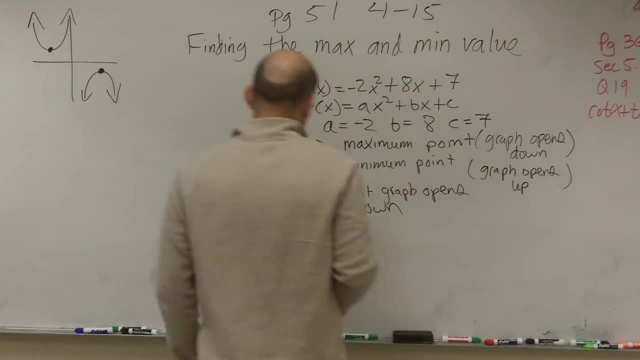 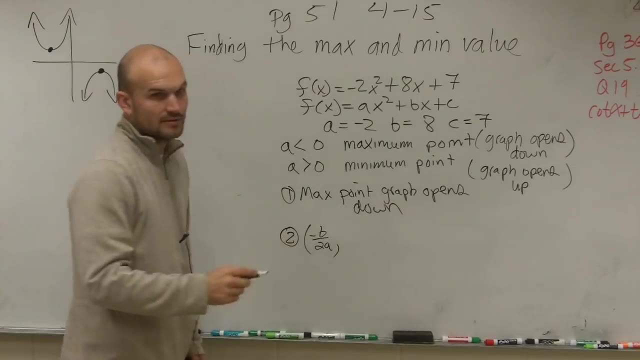 The vertex right. So do you remember the formula for the vertex is? it's a two-step process. The first point is opposite of B divided by 2A, right Opposite of B divided by 2A, which is our axis of symmetry. 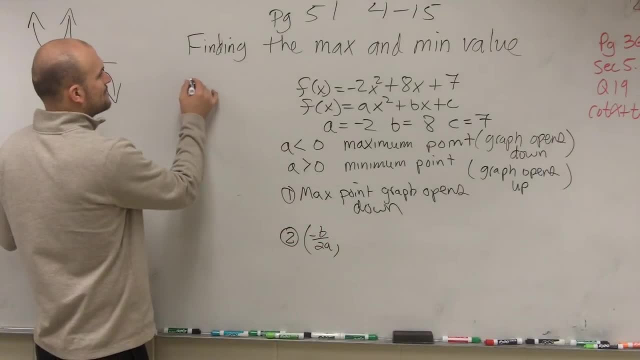 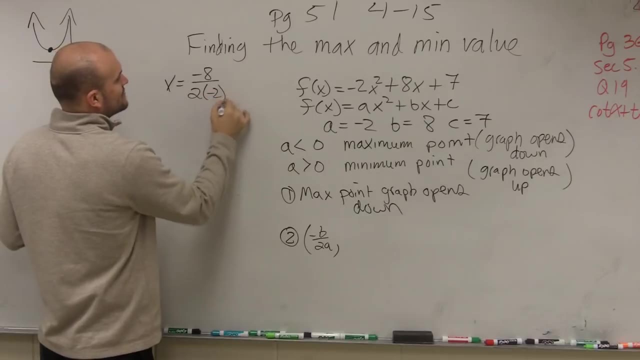 So this is actually kind of going back to the first problem we did. So what you do is you take opposite of, so X equals opposite of B, Which is negative eight divided by two times negative two. So negative eight divided by negative four is going to be a positive two.